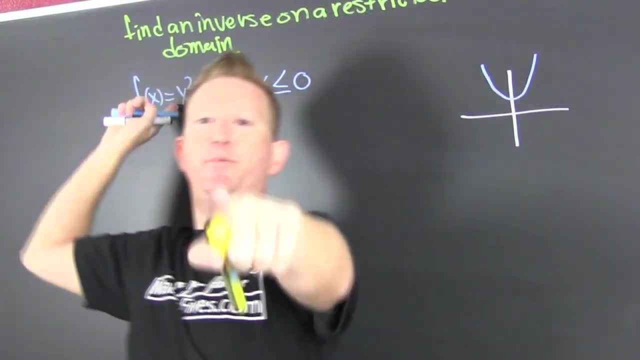 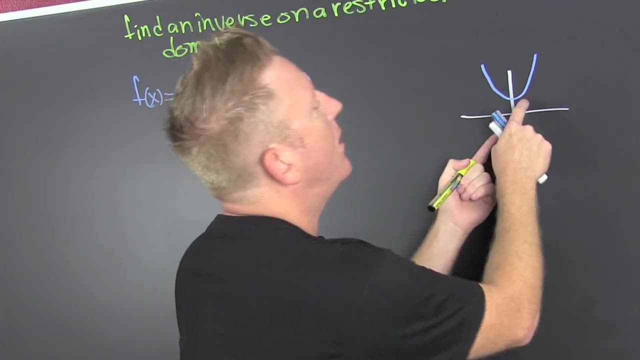 We want to go, and well, you get the picture. This is not a 1 to 1 function. That's the graph of that guy right there. Blue You, my boy. All right, It doesn't pass the horizontal line test, but what? 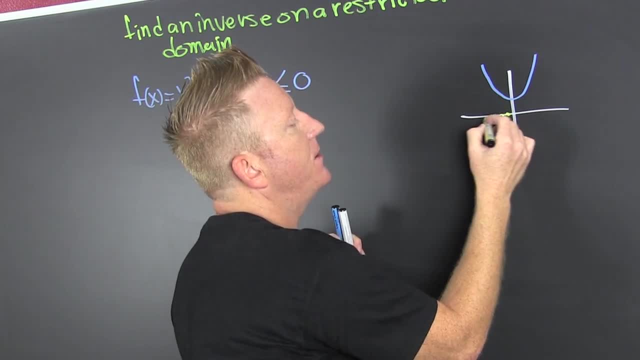 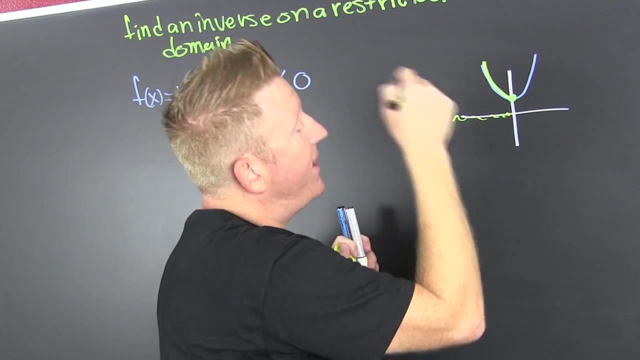 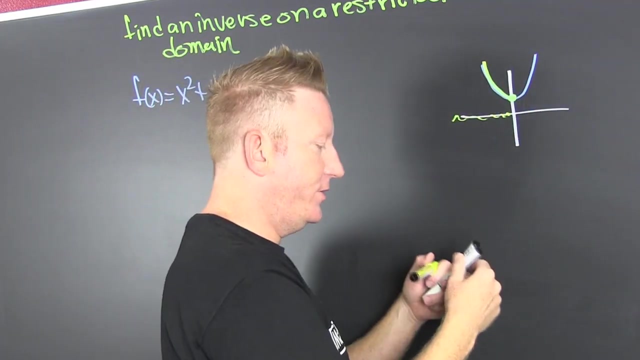 We have it restricted so that when the x's are smaller than 0, we only get this one piece. Now, if you consider this fine fellow, this yellow graph, then it does pass the horizontal line test, because we're ignoring your boy, So what? 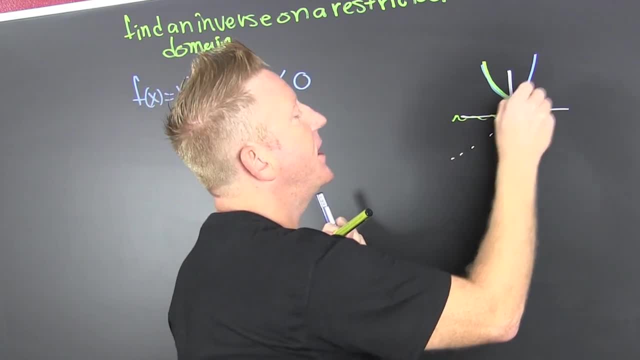 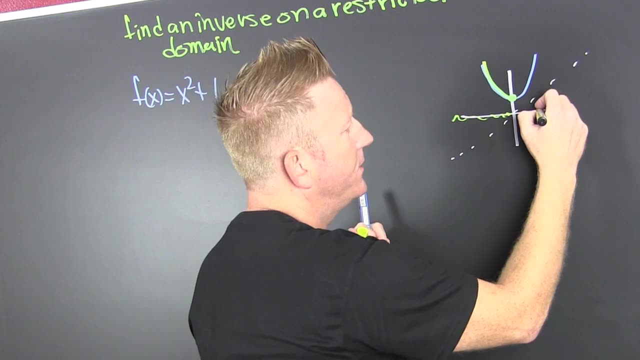 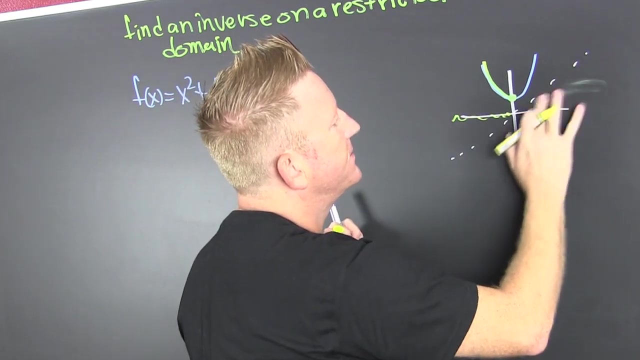 If you were going to go and reflect it across the line y, y is equal to x, then that's the graph of the inverse and it looks like it's going to look like: No, That ain't right, It's in the negatives. 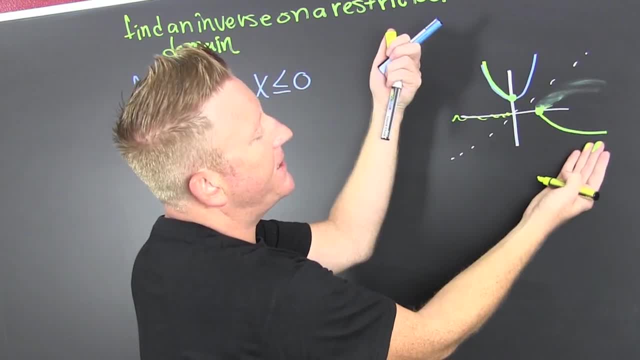 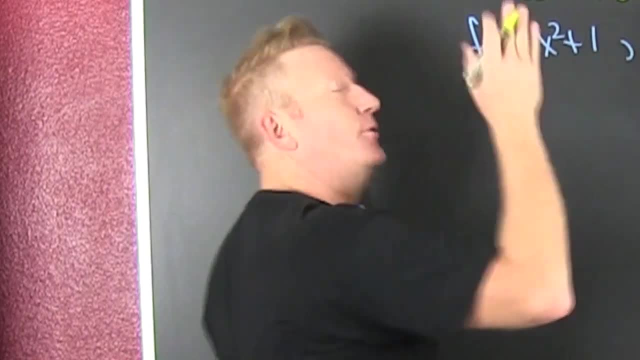 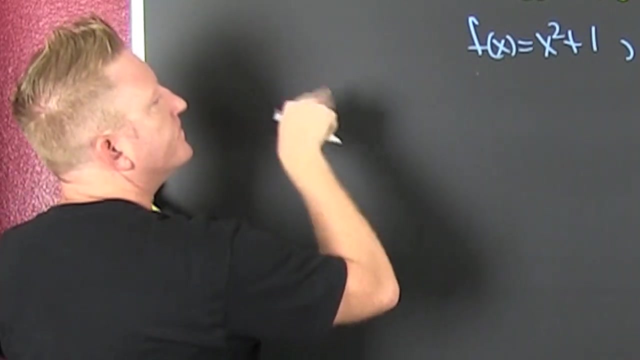 That's right. Right there, If I folded it, does it look like it's all symmetric? Sure, All right. So now let's go through that four-step process and, on the restricted domain, find- ah yes, the goods. 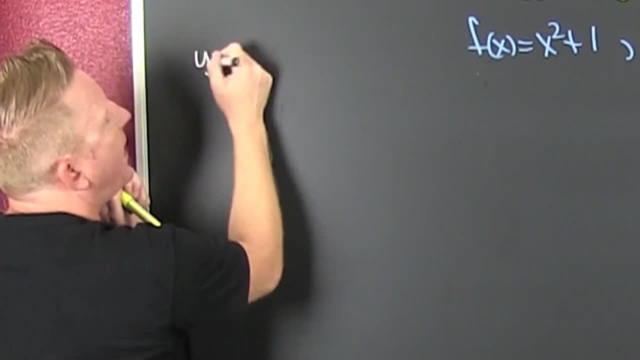 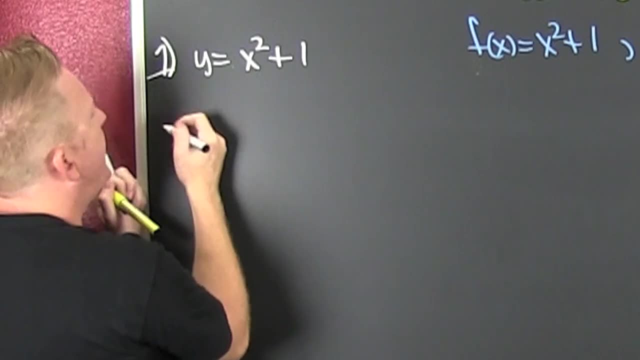 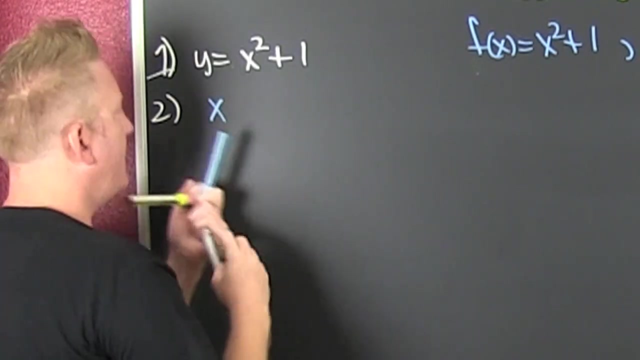 First step: replace f of x with y, Y, because it's easier on the i. that right there. That was step one. Step two: interchange x and y. Interchange x and y. So now I have my x is equal to my y. 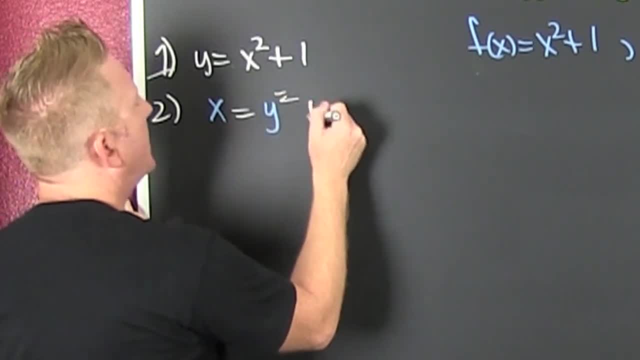 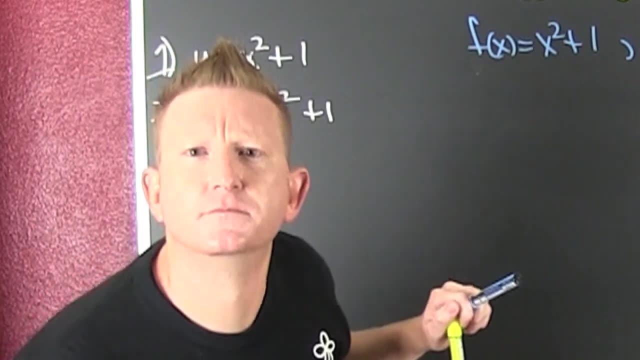 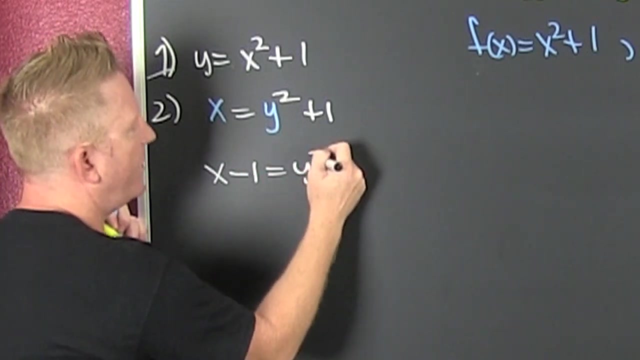 Square plus one. That's a deuce, All right. And now I solve for y, I do, and there it goes. So I have an x minus a one is equal to a y squared, All right. So now what? I take the square root of both sides. 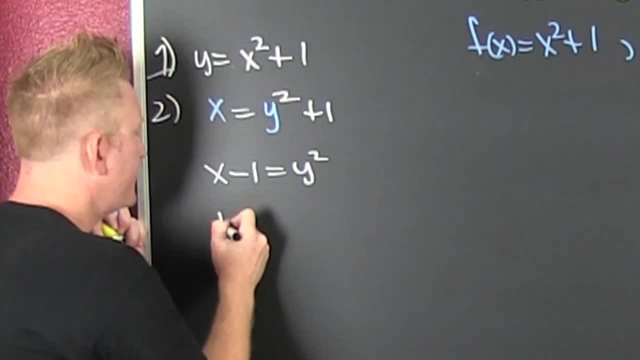 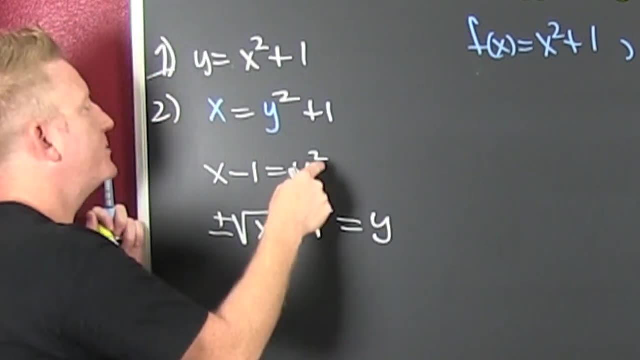 but I'm not going to forget the plus and minus. So that's plus and minus. the square root of x minus one Fun, That's going to be equal to y. Why? Because whenever I take the square root of ah square, you get the absolute value. 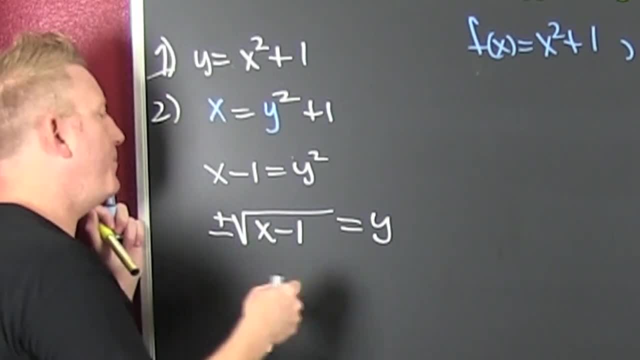 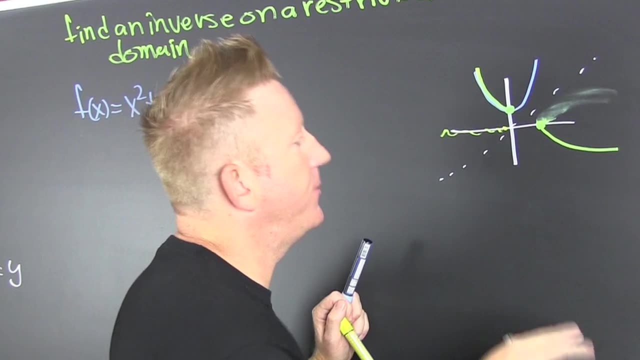 which is where the plus and minus come from. Now we need to pick one. Which? Which one Do we want the plus one or we want the negative one? That's where our picture is going to come out. It's going to help.